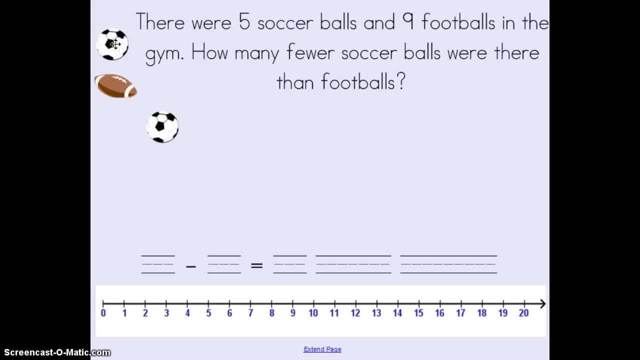 the slide. There were five soccer balls- One, two, three, four, five And nine footballs: One, two, three, four, five, six, seven, eight, nine. When I look at this picture, notice how I lined up each soccer ball with each football That way. 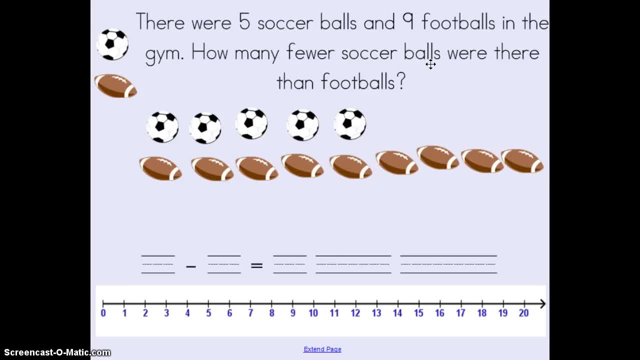 it's easier to figure out for the answer: how many fewer soccer balls. I can figure out how many soccer balls are missing to make it equal to how many footballs we have. Now it's time to write a subtraction sentence. Remember, in subtraction we always start with the. 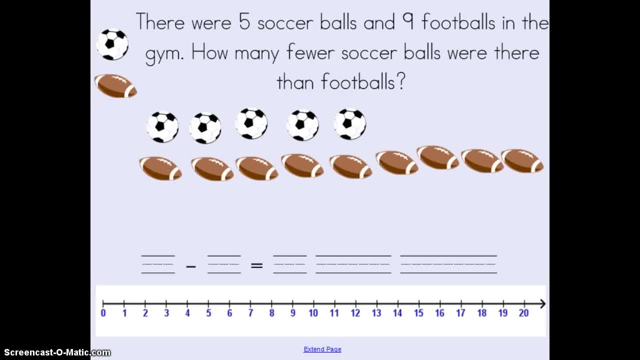 greater number. So in this case the greater number is nine. So I'm going to write the number nine minus. we already decided that for these problems, when it asks how many fewer or how many more, we have to use subtraction minus the smaller number, which is five. 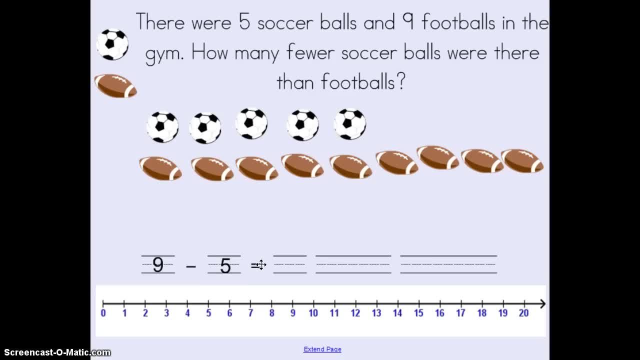 equals and we have to figure out the difference. Now, you can do this a number of ways. You can use the picture that I've put on here for you and figure out the difference between five soccer balls and nine footballs. Or you could use a number line, which I've also. 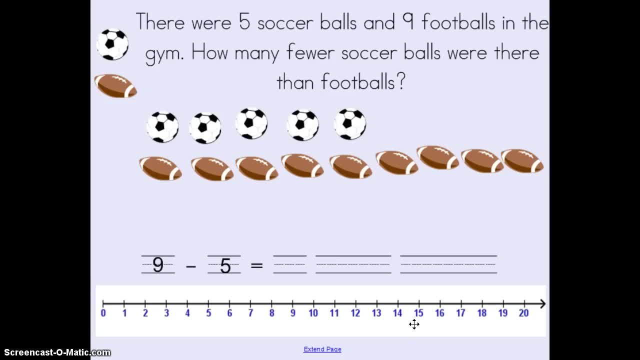 put on here Or any other strategy that we've learned for subtraction. I'm going to look at the picture and when I look at the picture, I notice that I have one, two, three, four extra footballs, which means I'm also missing four soccer balls. 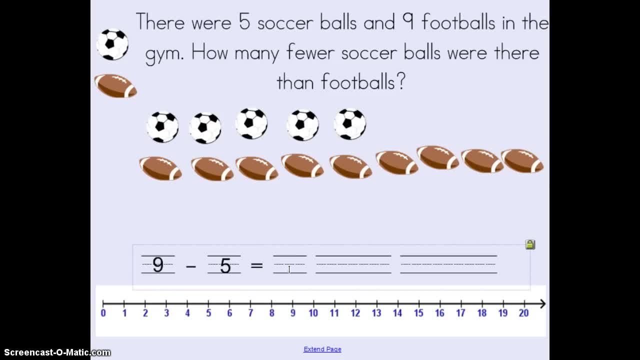 to make them equal. Therefore, my answer, or my difference, would be four. I'm also going to use my number line to make sure that my answer is correct, So I'll start at nine and I'll hop backwards five times: One, two, three, four, five Again. I land on the.